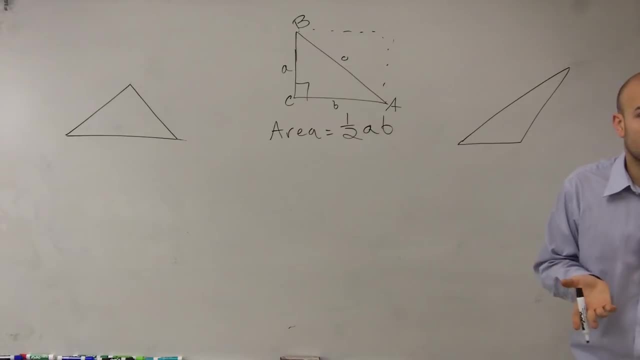 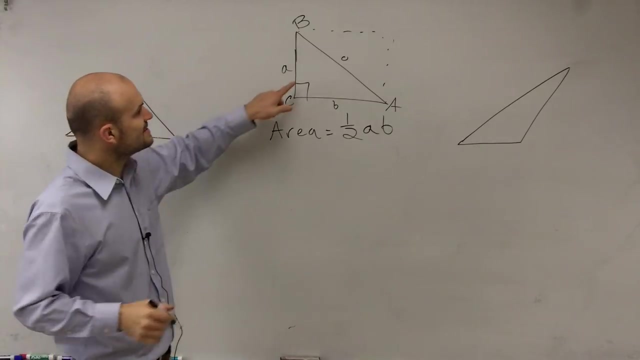 Well, first of all, we don't know what h is right. You're right, We need to figure out what the height is. So, in this case, we know our height is a because we have a right triangle and we have a right. 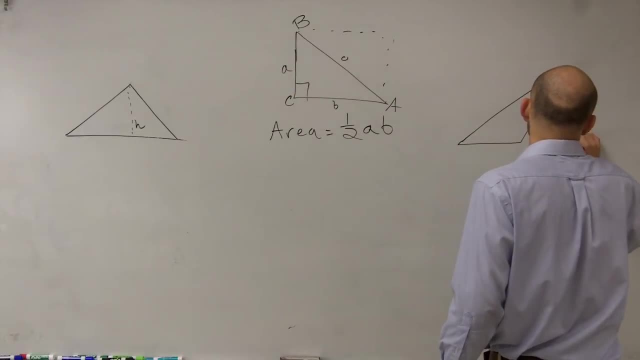 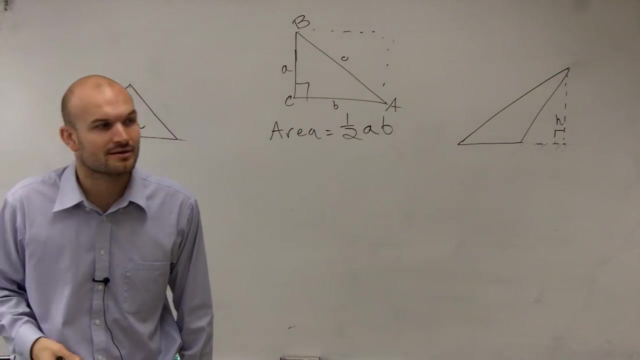 angle. so we're going to have a perpendicular line. So we're going to have a perpendicular line, but in both of these two cases you call this what. So we need to be able to determine. or do the Harlem Shake? we need to be able to determine. 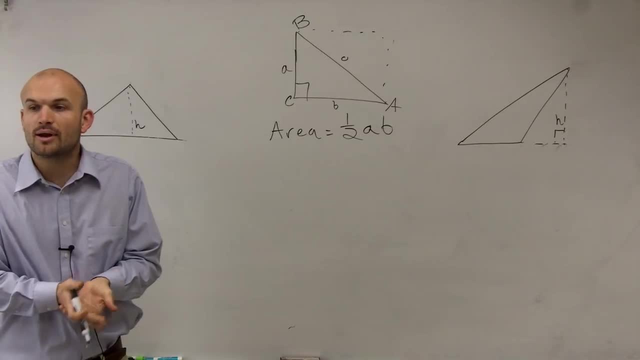 what exactly our height is going to be all right. So what I want to do is: let's take a look at how would we identify what exactly this sign would be if I said it's going to look like this, Let's see, Here's my angle. So if you have, here's my angle, a. 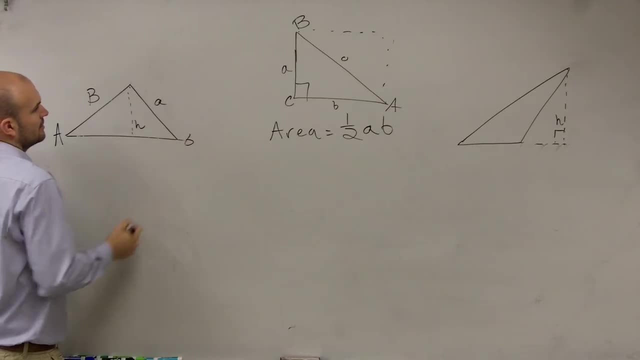 So here's the side length: a, b, little b, c, little c. So a What I'm just labeling my triangle, okay, So all I'm doing is I'm just looking at the triangle on how we'd go ahead and complete it. I just want to make sure using my b across from there. So if you guys are looking at, 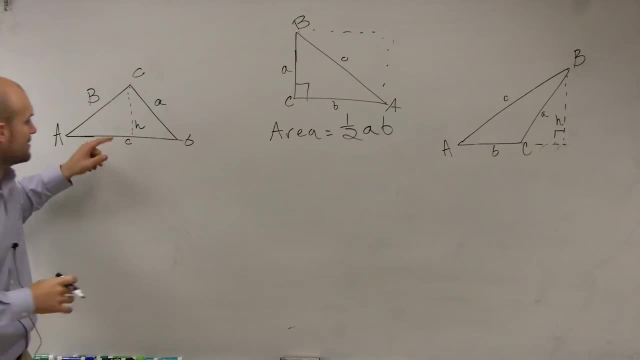 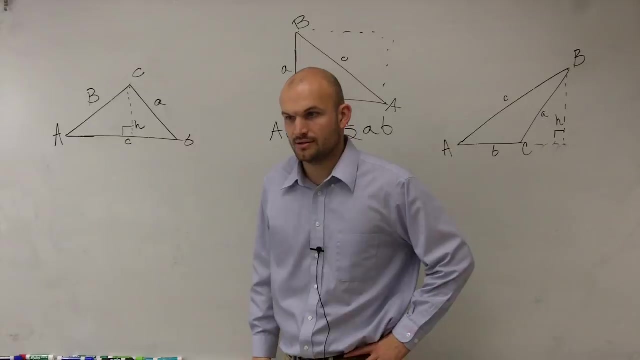 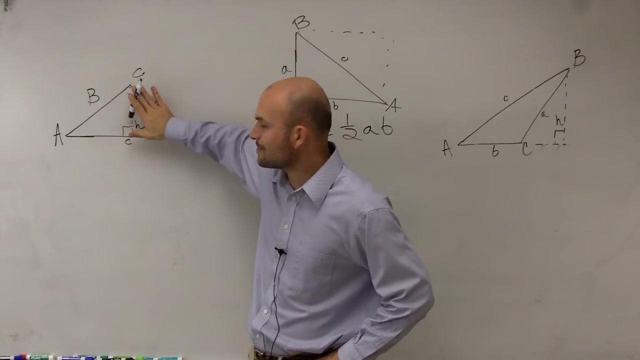 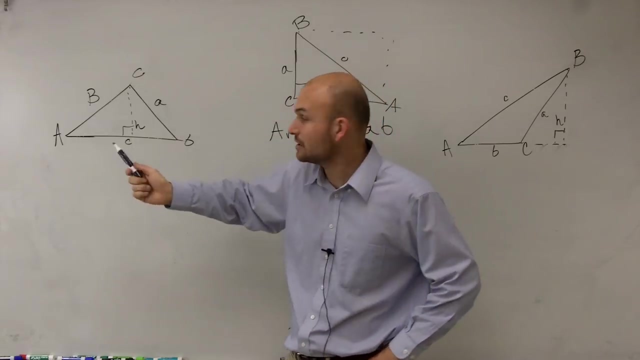 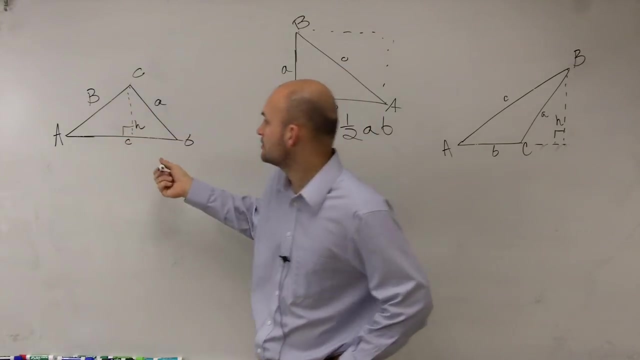 this: if I want to find the length of my a, all right, I'm sorry, I need to find this height. Let's pretend I create a right triangle with this right. So now I can say: how would I be able to figure this out? Well, I could say that the height of this. if I was going to kind of break this up and just look at this from a right triangle standpoint, I could now say that now, knowing what sine cosine tangent are, this h is equal to the sine of a, which is opposite. over smaller case. I rewrote those. 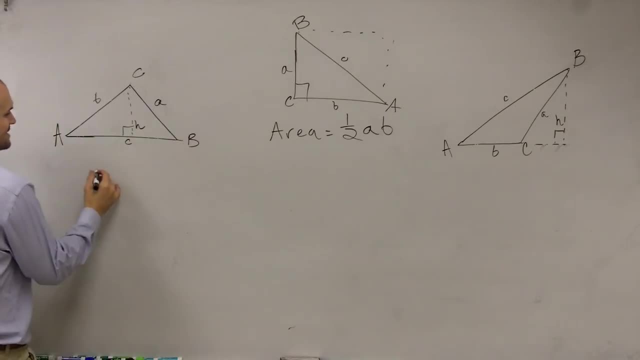 So I could say that the sine of a is equal to h Right, And then, if I just want to figure out what h was, I would multiply b on both sides and therefore I could say h equals b times the sine of a. 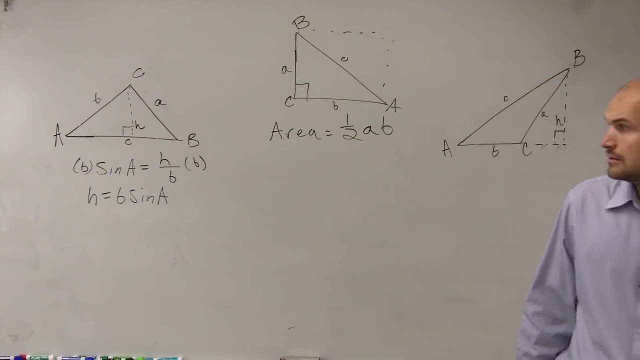 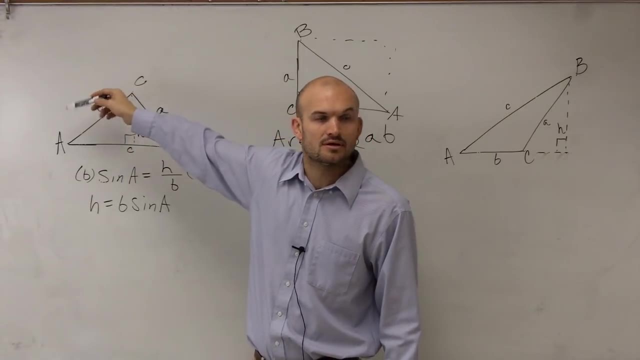 Does that kind of make sense? what I did? Because remember, if I wrote this triangle, remember sine is opposite over hypotenuse. So what I did is I created a right triangle. right, Because we can only use our trigonometric formula. 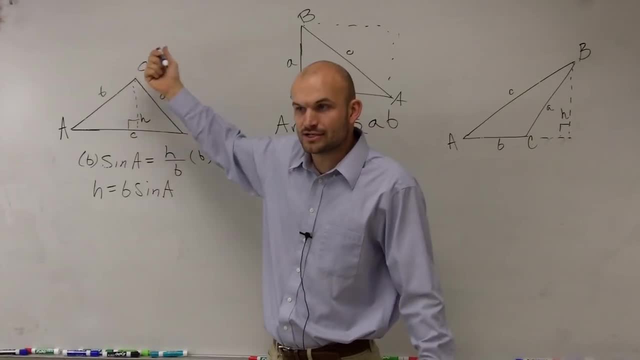 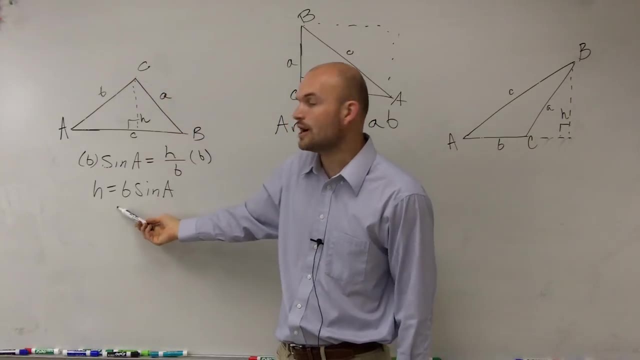 We can only use our trigonometric formula if we have a right triangle. So what I did is I created my own right triangle. so therefore I could say, oh, hypotenuse is or sine is opposite over hypotenuse. and now, by solving for h, I can say: oh, the height of this oblique triangle is b times sine of a. 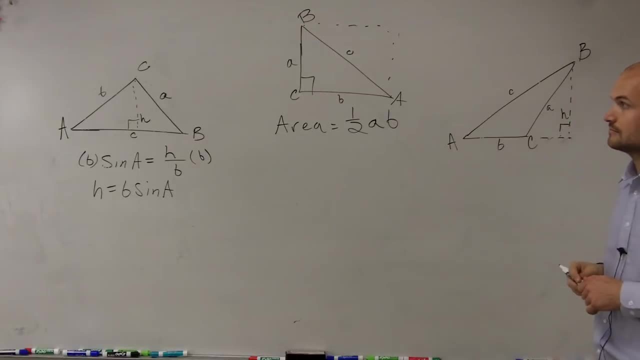 Yes, Um, are you trying to find the height? Are you trying to find the area of both triangles? No, I'm going to show you some formulas that we're going to use Right now. I'm kind of explaining why we're able to do this. 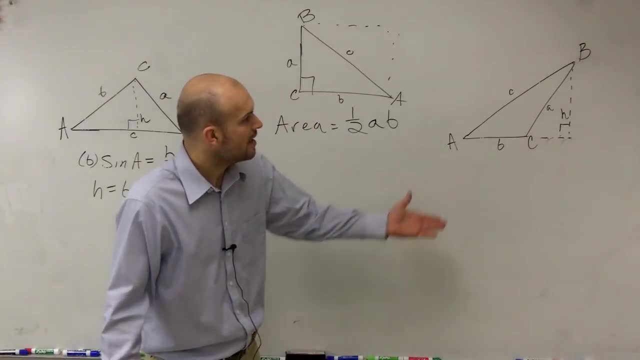 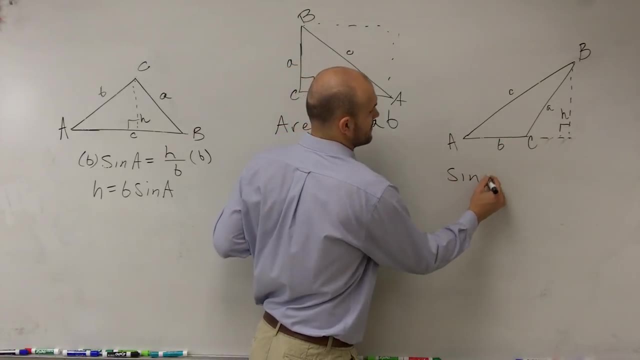 I'm explaining why h is going to be equal to this and why it's going to make sense. And then over here, if I wanted to find this right, if I wanted to find this height again, I'd use: sine of a is equal to h over c. 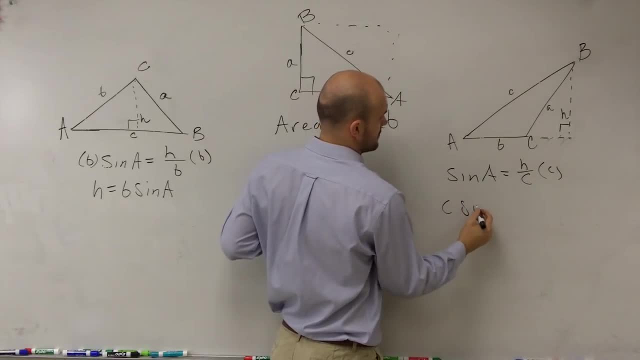 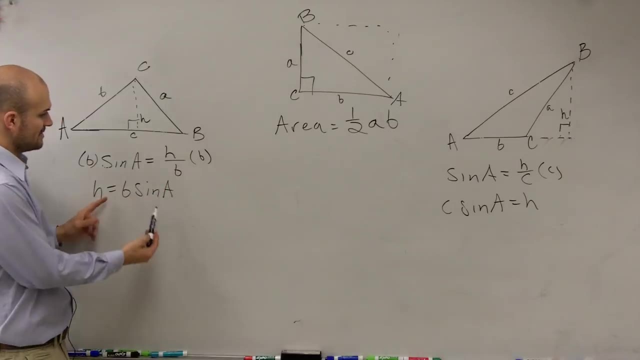 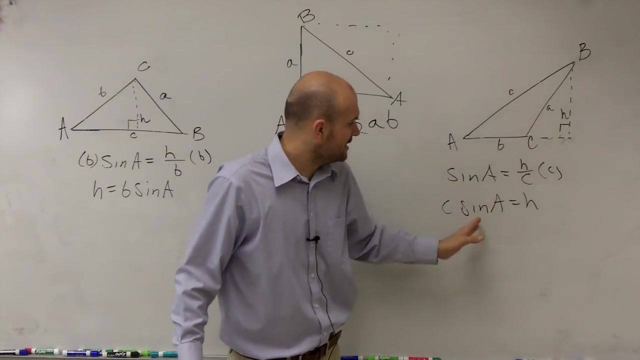 Again solving for h. So, as you guys can see, it doesn't matter. it's not going to matter what, if it's, what kind of triangle I'm dealing with, but your hypotenuse or your h, your height, is always going to be one length times your other length, right? 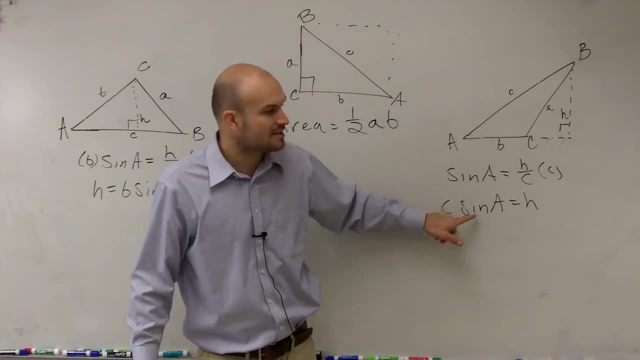 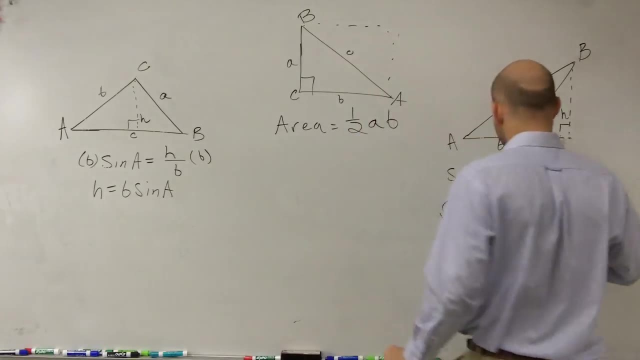 Or I'm sorry one, your one length of your triangle times your height. Or, I'm sorry, here is your height, which is going to deal with the sine of your angle right times another length of your triangle. Now, remember, we talked about length. so if let's say that's your height, right? 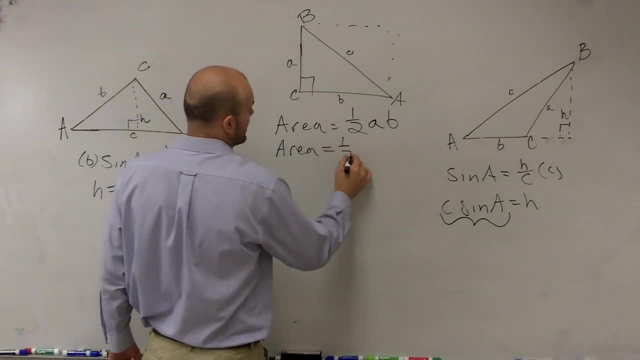 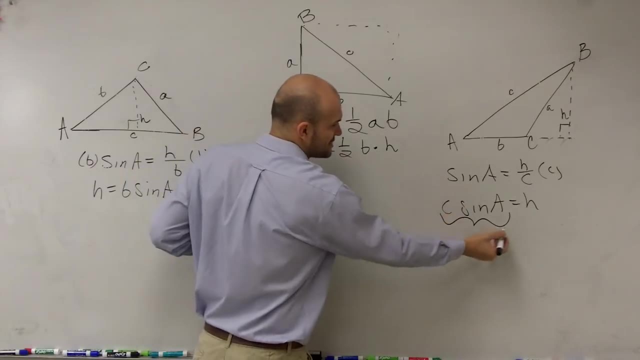 Because we said area- let's rewrite this in different- is one half base times height, right? That's another way to kind of write it. Well, we already know what h is right, So h is this. So therefore, let's say, pretend I know what my h is.